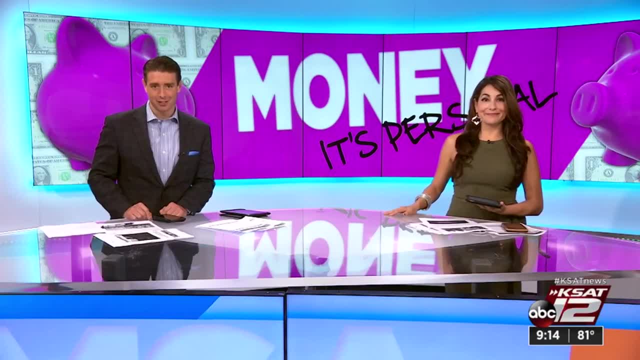 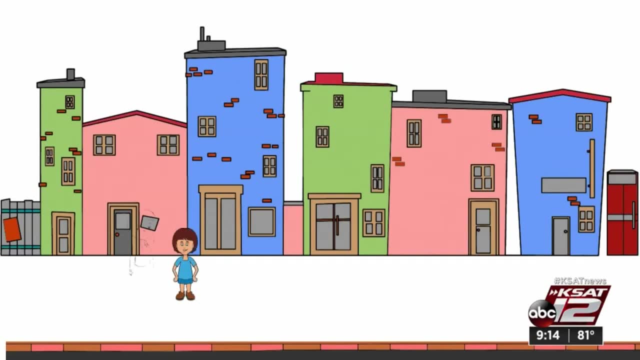 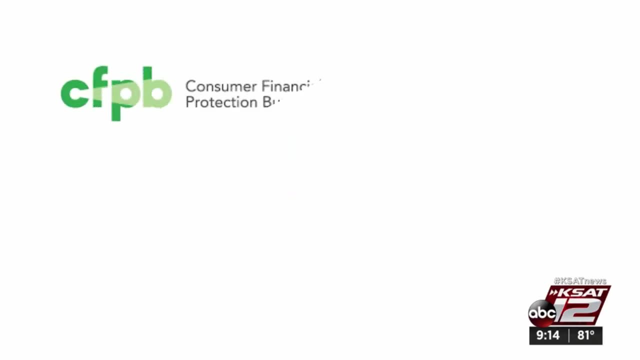 have conversations with your children about shopping responsibly. Anne is four and her big sister, Diana, is 11. They're learning how to shop responsibly with the help of their dad, Andrew. The Consumer Financial Protection Bureau is offering families like theirs some tips to help them discuss ways to spend money wisely. Andrew can show little Anne. 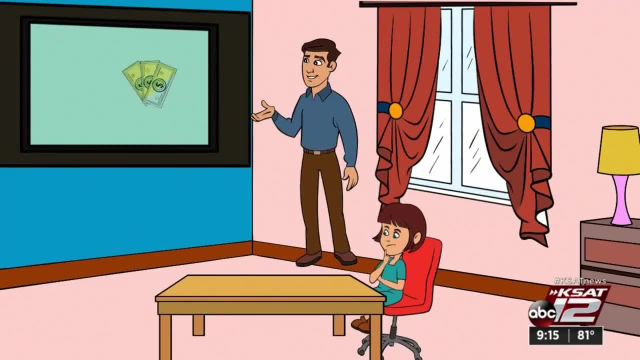 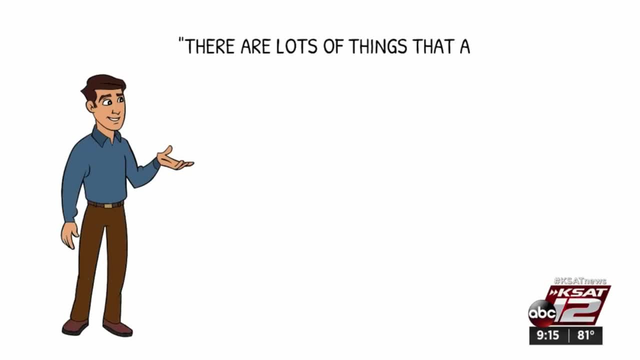 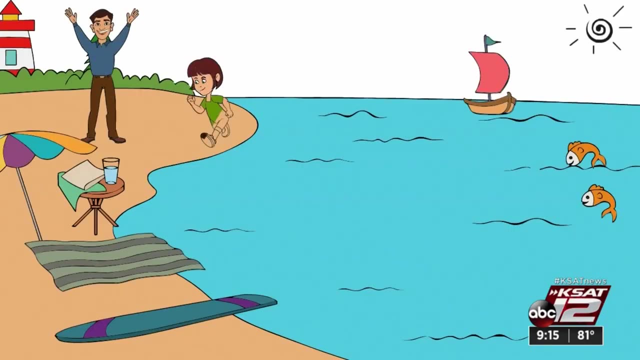 the different types of bills and coins that exist, so that she can learn about the currency she will one day use to pay for items. Andrew can also use a phrase like: there are lots of things that are of value and some of them cost money. Anne's dad can give her examples about the free things in. 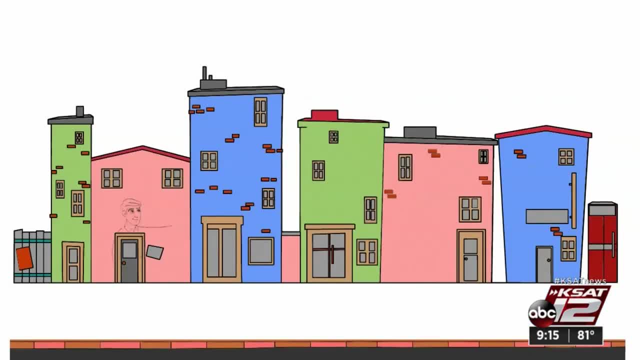 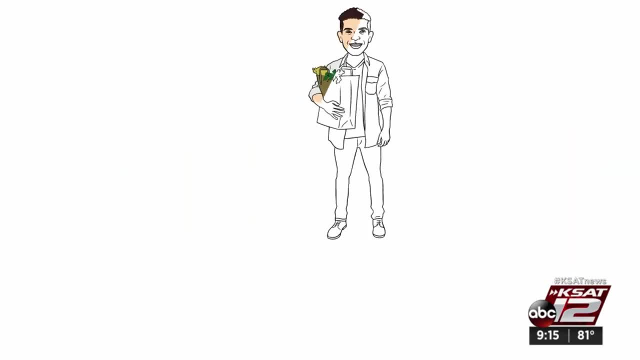 life, Like spending time with family members, And he can talk to her about things that cost money, like school clothes or gas. Anne can also learn about the choices one has when they're out shopping. Andrew can use real-world examples to help her understand this concept, like explaining. 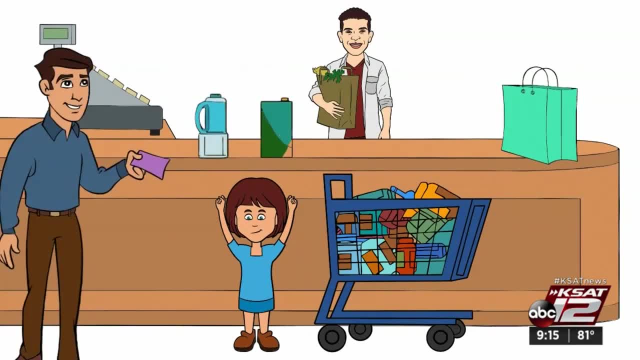 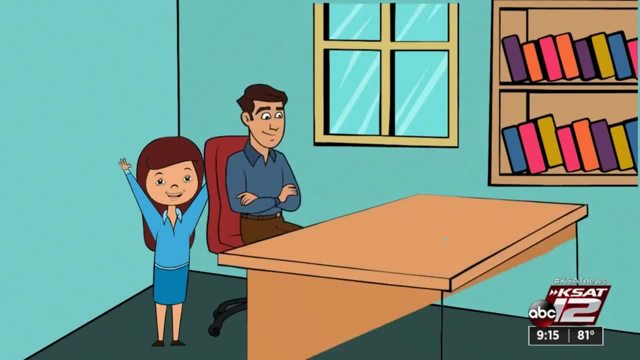 the family budget, or why he picks one item at the grocery store over the other. Now, since Diana's a little older, Andrew can discuss cost-saving shopping with her and also warn her about some of the hurdles she may have to face, And he can also teach her how to shop responsibly. 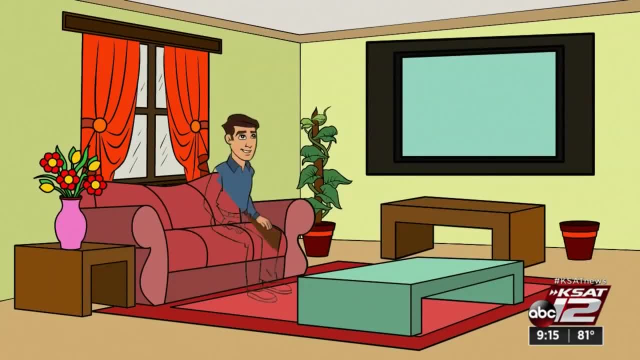 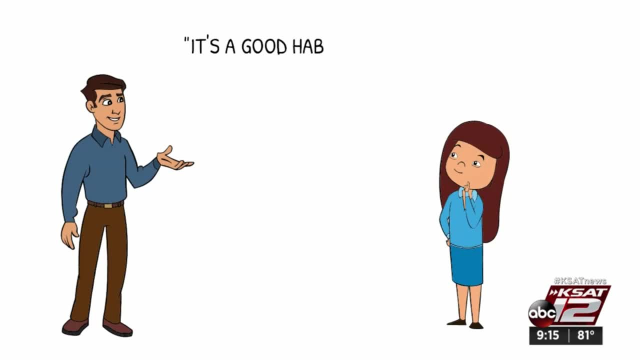 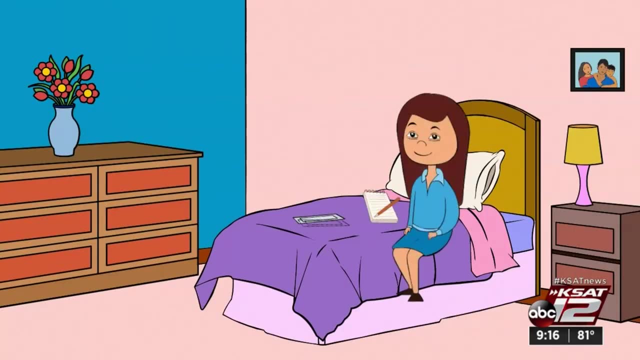 Andrew can talk with Diana about advertising and how it can get people to spend more money than they anticipated. Andrew can use a phrase like: it's a good habit to shop around and compare prices before you buy. This can help Diana understand how to shop wisely. Diana can also learn about 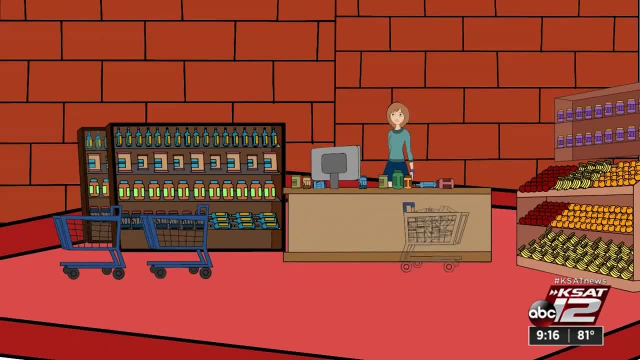 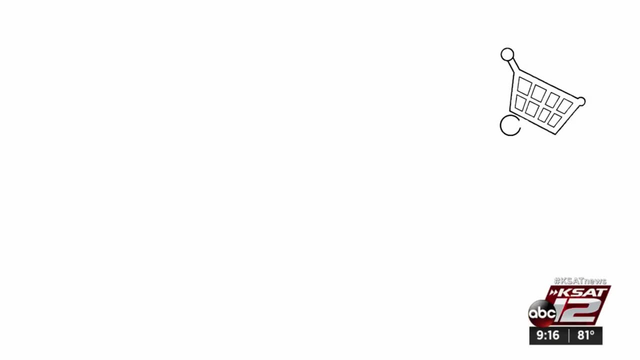 how to use coupons or discount codes. Andrew can point out the savings he gets in the real world or while shopping online to help her understand. Andrew can also use some of the resources he has to spend to buy a few things. He can also learn how to use a coupon or discount code. Andrew can also 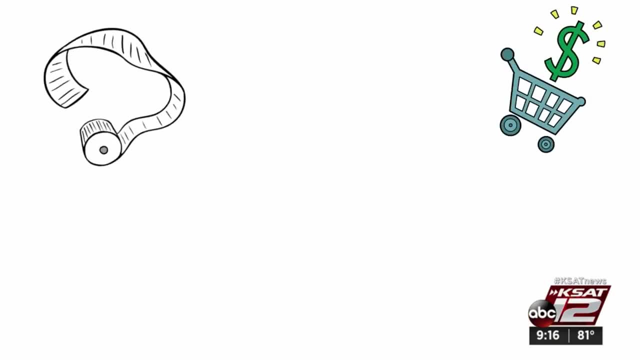 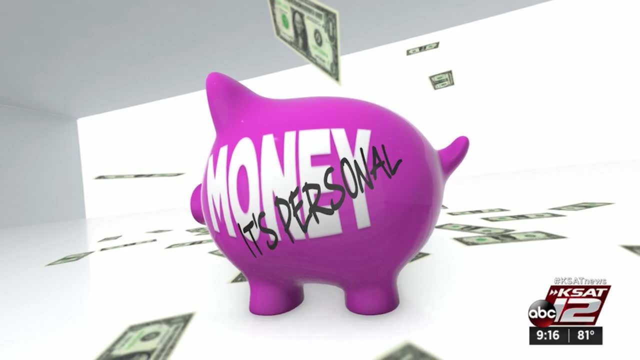 Store receipts to help Diana understand the concept of sales taxes and how to plan for them. For this week's Money is Personal. I'm Ivan Herrera KSAT 12 News And we have a link to those tips on our website right now. 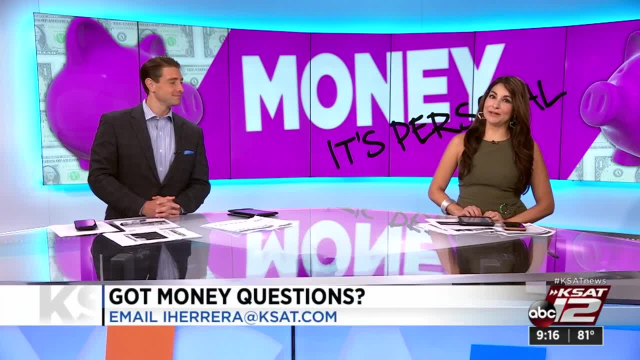 Just visit ksatcom, slash MIP And if you have any money questions, you can submit them by emailing Ivan at the email at the bottom of your screen.